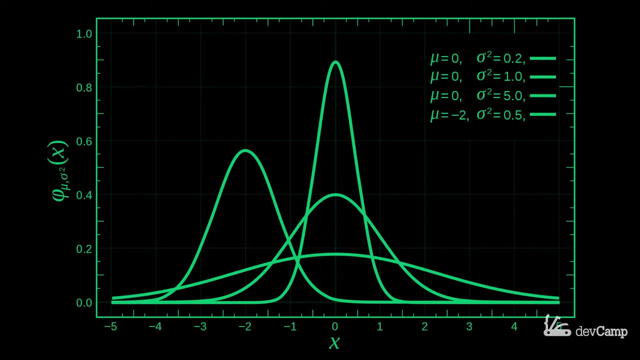 directly, but instead they are the different parameters that, once they've gone into the algorithm, they were generated, such as the standard deviation, And so those were used in order to build out that training model. So right here, as you can see, with these set of graphs, 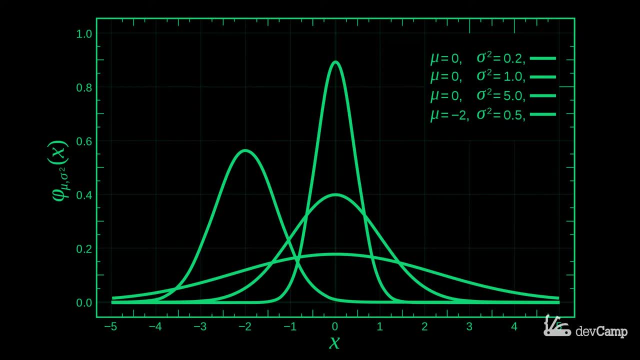 we have four different types of parameters. We have means that range from zero to negative two, and then we have standard deviation, going from point two all the way to point five, And then when you place those inside of the algorithm, then it generates these various 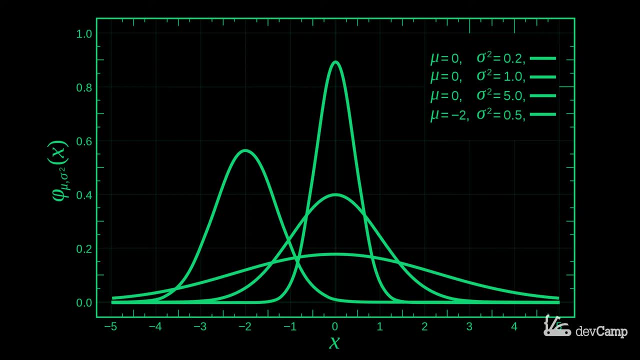 curves, And so you don't have to worry about the graph. in this sense, I want you to just focus on those items on the top right-hand side, because those are the model parameters. They're what are being used in order to generate the different linear regressions. 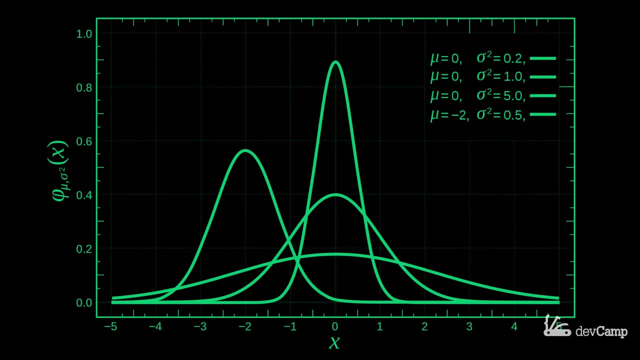 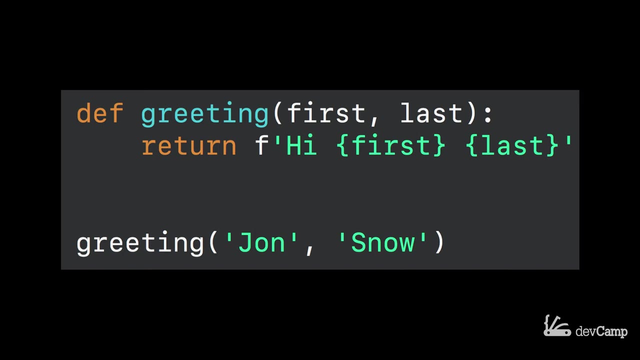 or whatever type of algorithm that is being generated. Now, that is a model parameter. Now, if that is still not perfectly clear, let's look at a programming example, Because in programming such as in Python, Python functions have parameters. So right here we have a basic greeting function. 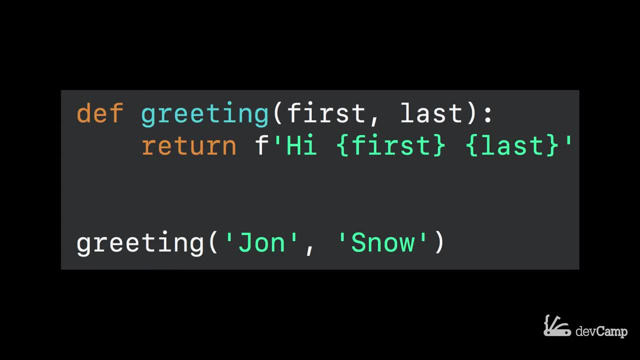 and the greeting function takes in a couple arguments. It takes in a first and a last name for arguments. But then when we call that function- so when we call greeting down on the bottom, we pass in two parameters. We pass in John and then Snow. 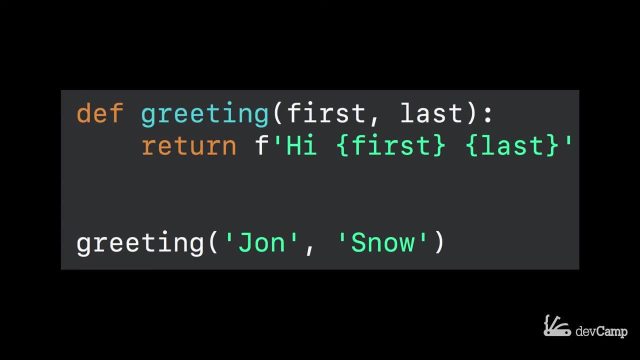 and then those parameters are used in order to return the value. Now, this is a very basic example, but this may also help you to understand exactly how parameters are used, even in a slightly different way than they may be used directly in machine learning. So those are model parameters. 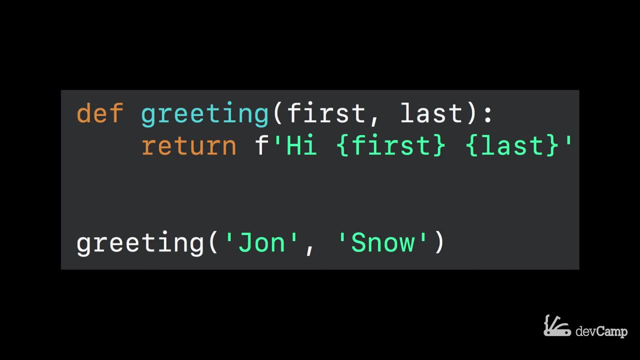 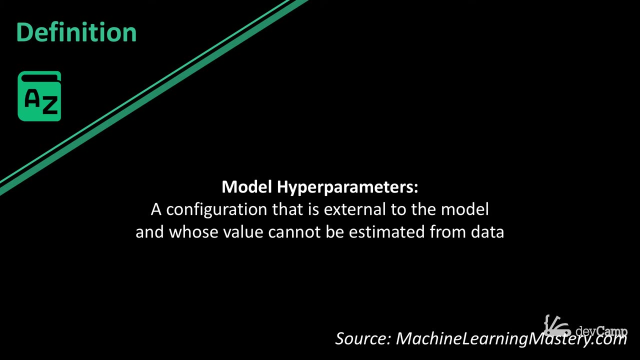 They are the data that you're working with and they are the different elements that are generated from the machine learning training data set. Now let's talk about hyperparameters. So, when it comes to model hyperparameters, the definition for that is that it is a configuration.